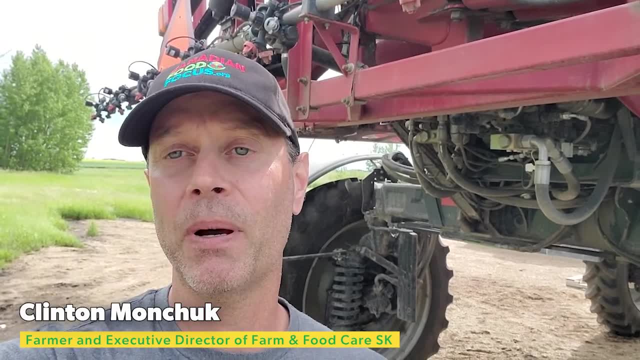 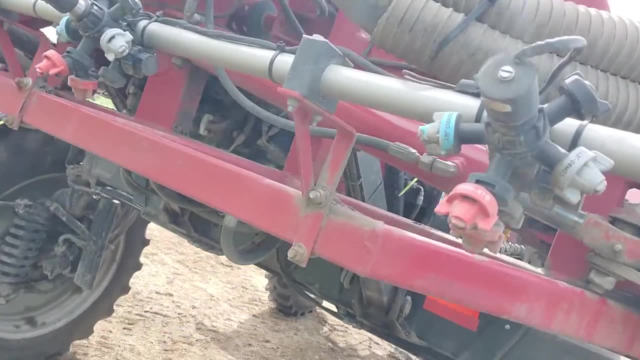 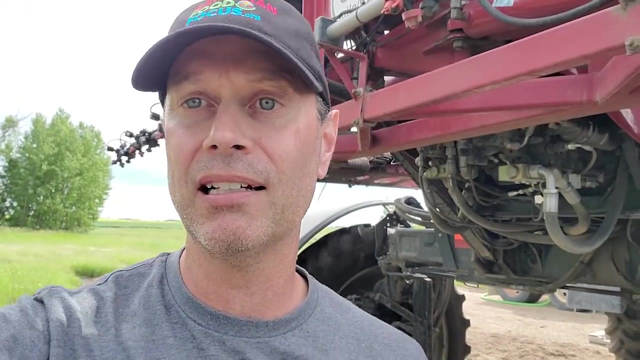 from five gallons an acre up to 20 gallons an acre, depending on what we're spraying in the field for herbicides or fungicides or insecticides. But everything is controlled with this. So that is a solenoid and it goes back to a GPS system in the kind of the main computer of the sprayer. 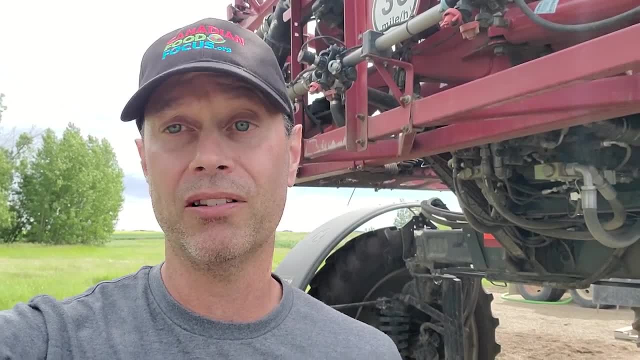 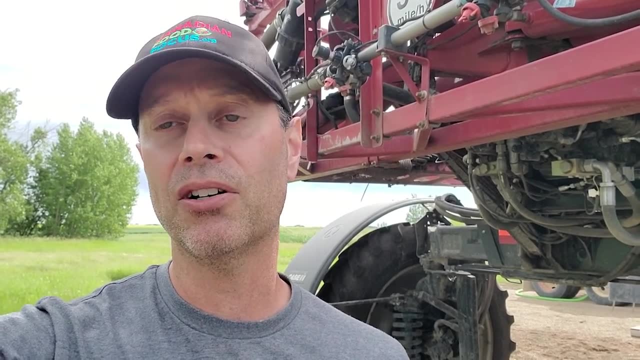 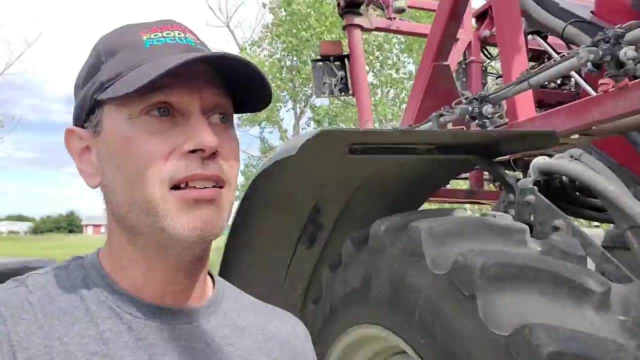 and it automatically turns on and off depending on where you are in the field. So that's so we don't over apply any of the the herbicides or fungicides and make sure we're saving money really with what we're doing. The other thing that I want to mention is that this is pretty big, so I'm 6'3 and this is a pretty 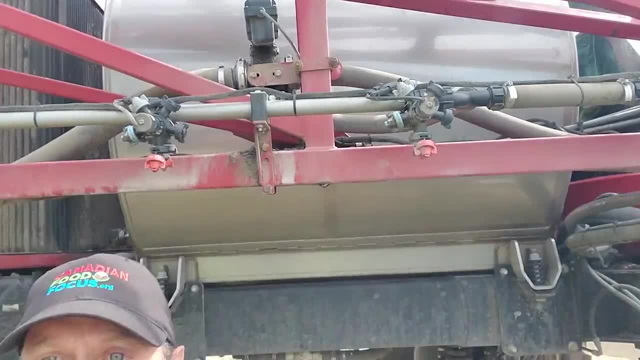 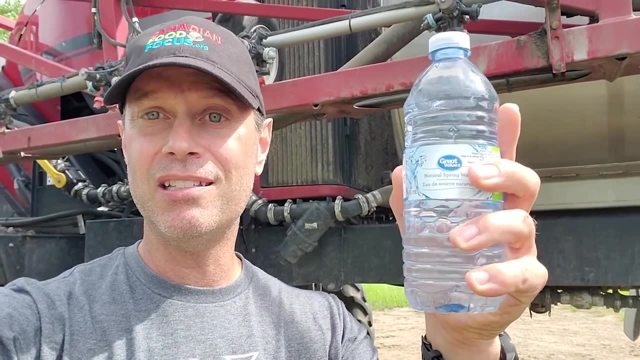 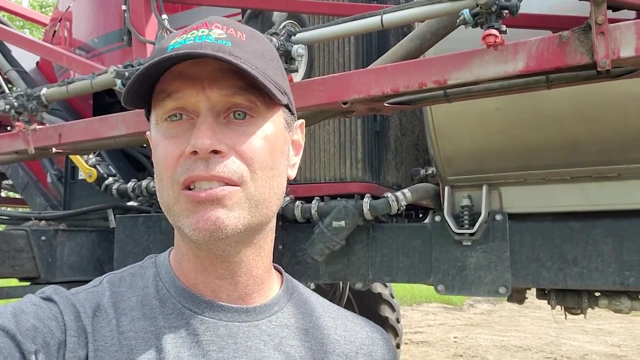 big sprayer, That silver thing, that's the tank, and it holds about 1,200 gallons. Now, majority of what we spray is actually water, So this is a half a liter bottle of water Effectively. most of the herbicides are fungicides, So this is a half a liter bottle of water Effectively. most of the 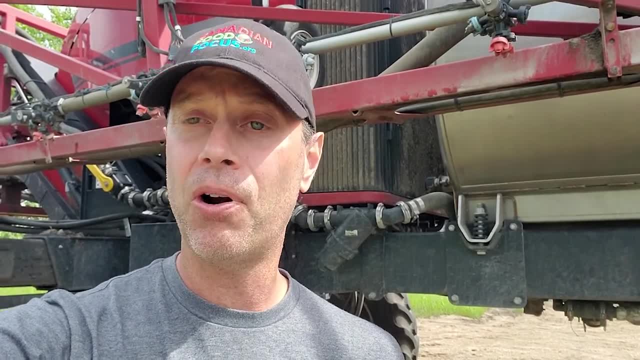 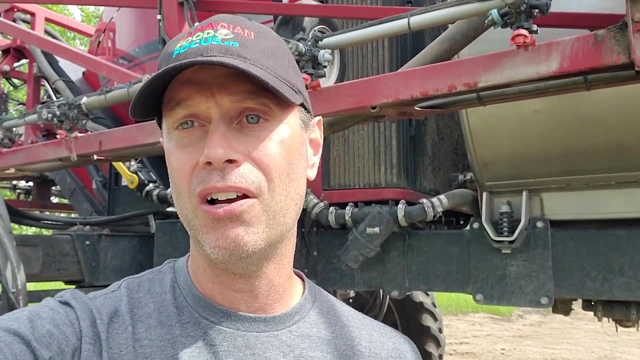 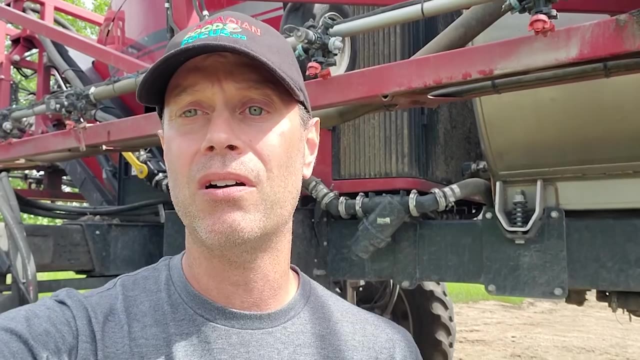 fungicides we use are kind of around that half a liter per acre. An acre is roughly the size of an American football field. So it's very small amounts of the herbicide or fungicide that we put on and they're very targeted to just target that disease or that weed or that group of weeds. 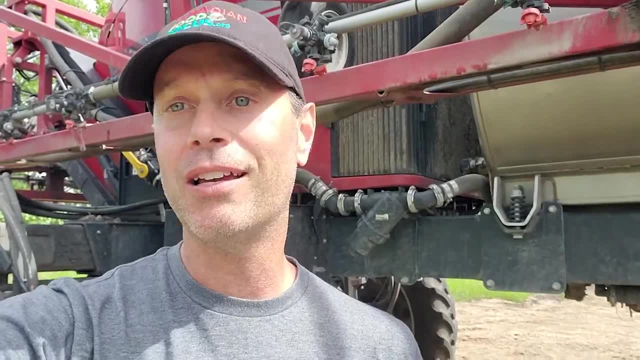 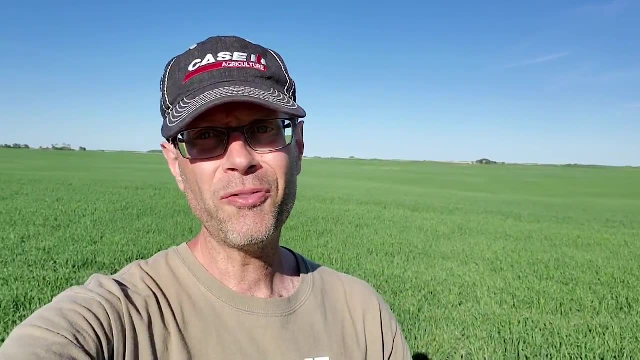 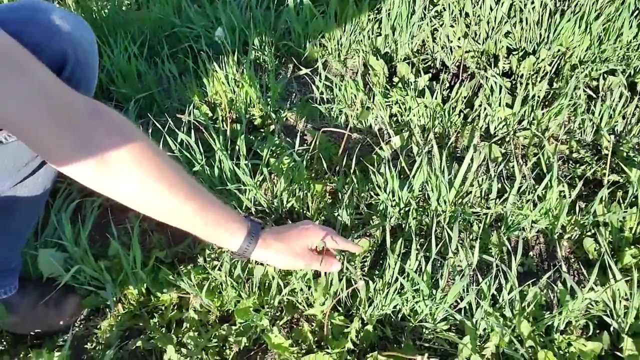 that we're trying to kill to make sure we have healthy wheat and barley and oats and canola and corn and soy and all the other things that we grow here in this wonderful country. In a perfect world, our crops would be planted and only these things would grow instead of these. 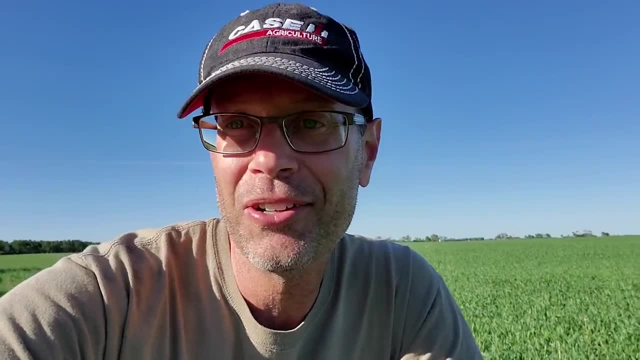 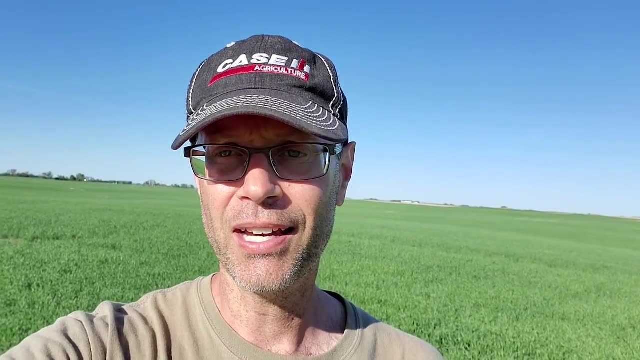 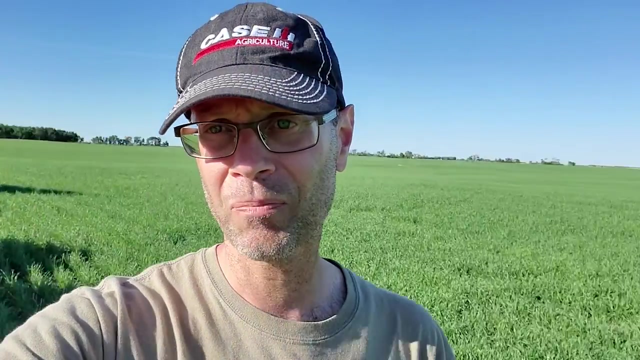 things. These are weeds. Well, weeds take all the nutrients away from the plant that we want. So in this case there's barley in the field, So we don't want that. We want to make sure that it's only barley growing out here, and you can see this is one small field. It's about 110 acres, 110 football. 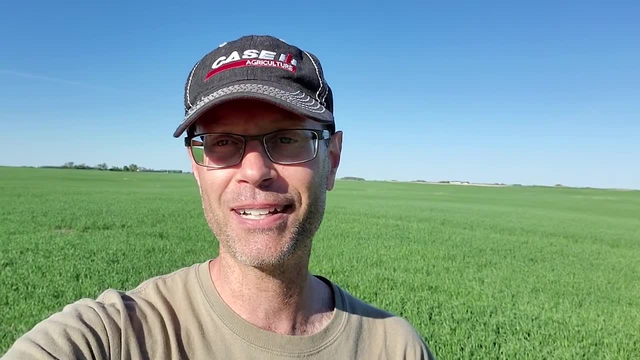 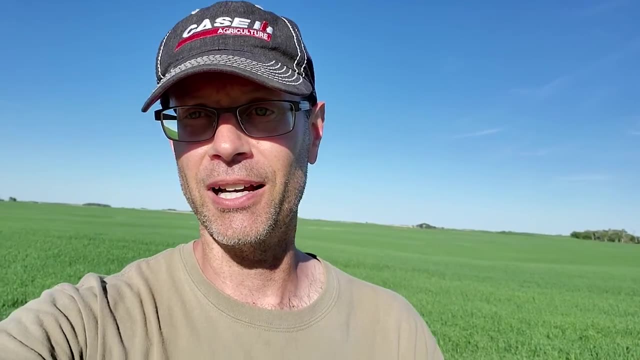 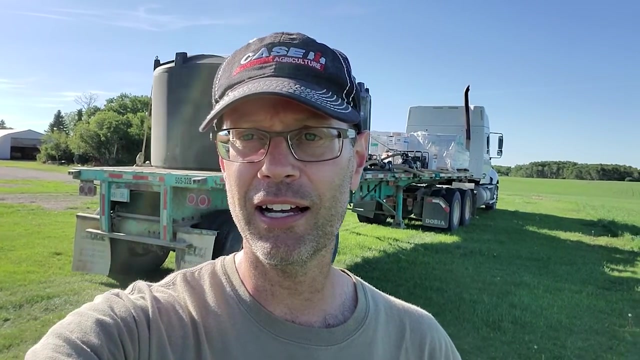 fields. So you can imagine if we had to pick this all by hand my back would be even more sore than it is already. So we have to use herbicides to spray them, and my brother's just coming in with the sprayer- in a bit I'm the water boy today. So we have the two big tanks of water and the herbicide.